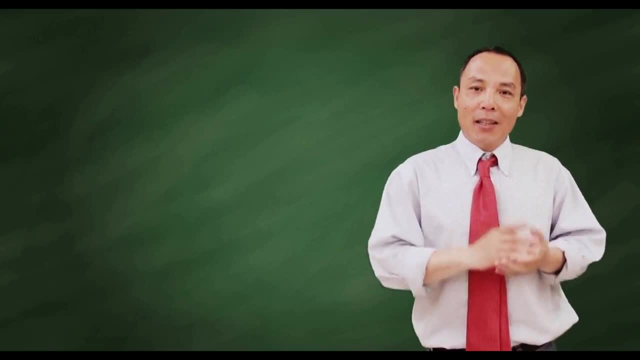 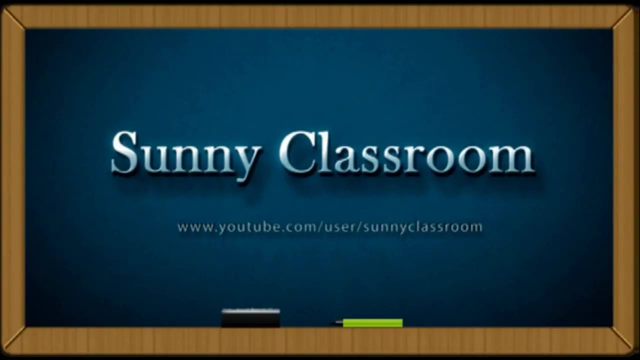 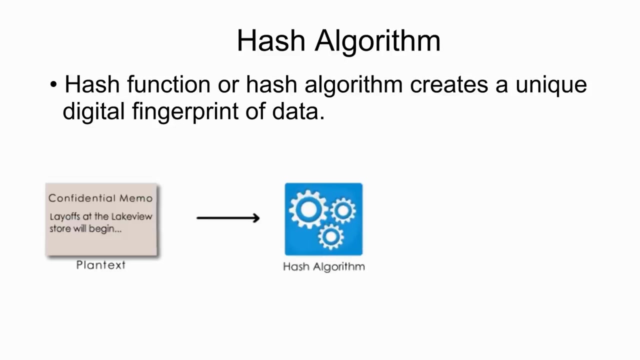 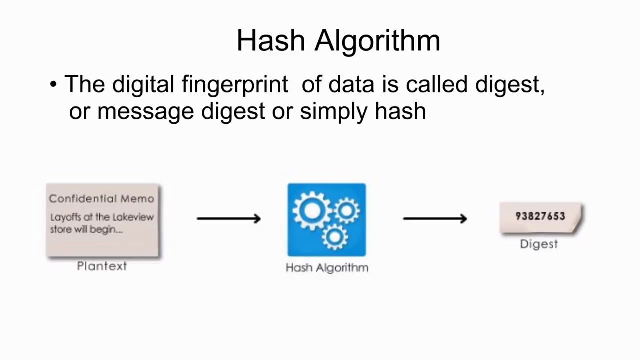 Hello, this is Sunny. Welcome back Today. my topic is hash algorithm. Hash function or hash algorithm creates a unique digital fingerprint of data. The digital fingerprint of data is called digest or message digest, or simply hash. Hash algorithm is primarily used for comparison purpose, not for encryption. 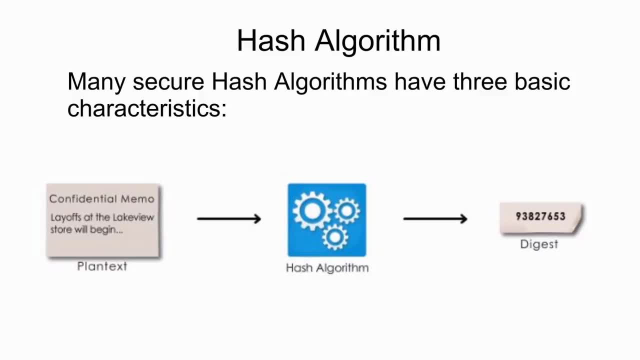 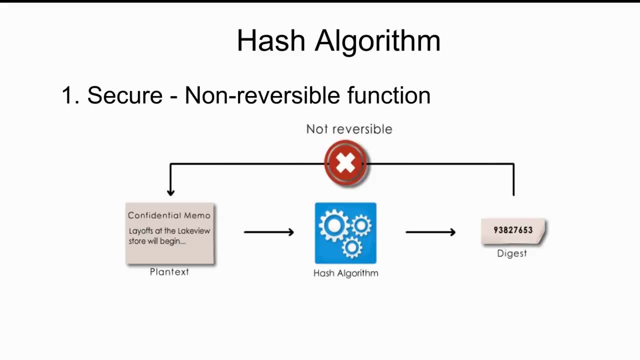 Many secure hash algorithms have three basic characteristics. One: secure Results. Resulting hash or digest cannot be reversed to determine original data. Hash algorithm is not reversible. It's one-way function. Given a digest, you cannot get the original data. 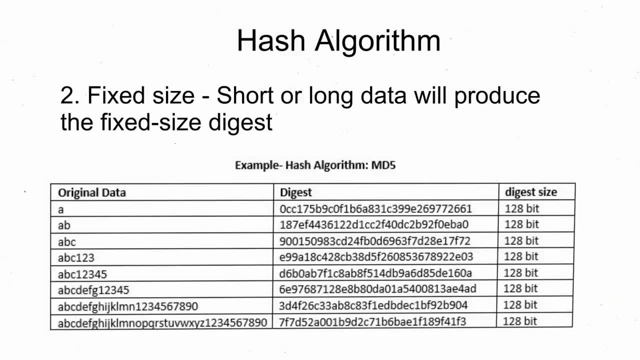 Two fixed size. Given a hash algorithm, you will get fixed size digest, no matter how original data varying length, Short or long data sets will produce the same size digest. Three unique, Two different data sets cannot produce the same digest. 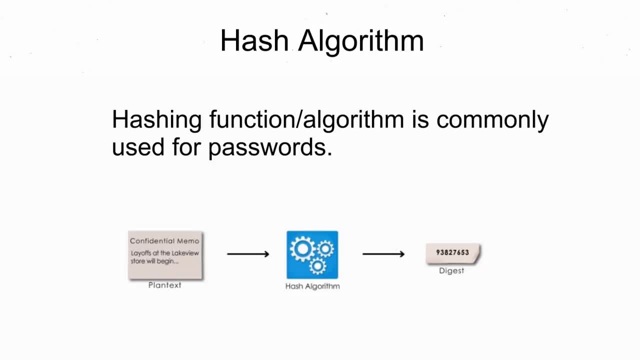 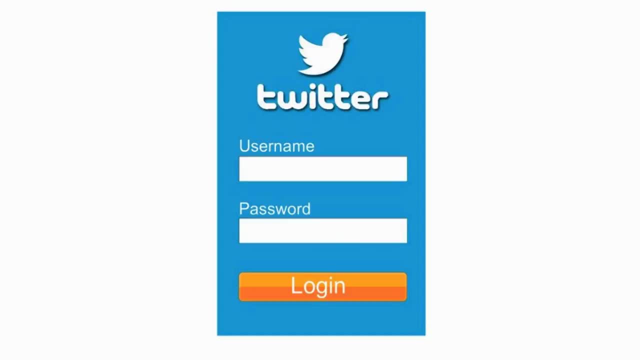 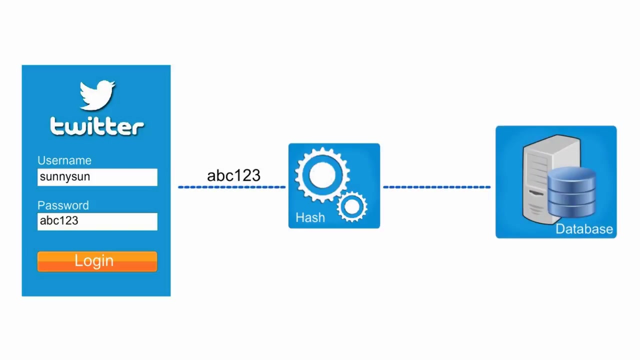 Hash algorithm is commonly used for passwords. Take Twitter as an example. Today, I want to see what's going on with Donald Trump. I need to log in first my username, signing sound my password: abc123.. When I click, submit both my username. 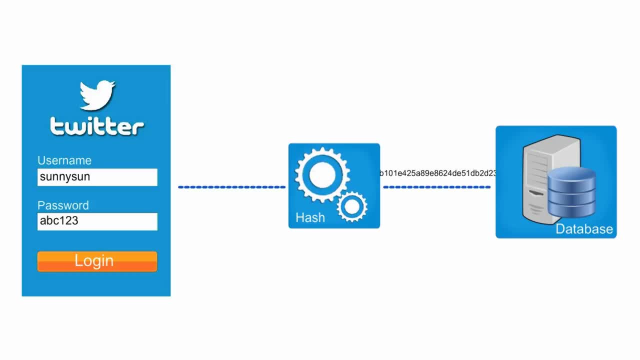 and password would be sent to Twitter database. But before my password is sent to the database it is hashed to a digest. Let's assume Twitter use SHA-256 as their hash algorithm, then my password digest would be 256-bit long. You might say, hey, your password is too easy.